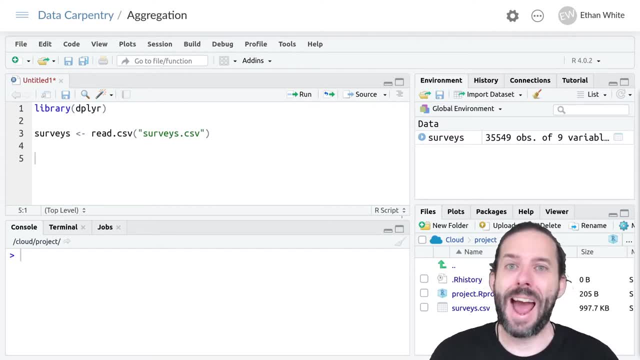 So, for example, if we wanted to calculate the average weight of an individual in each of the different species in our data set, we could do that by aggregating the data. The first step in this process is to group the table so that it knows what the groups are to do. the calculations on: 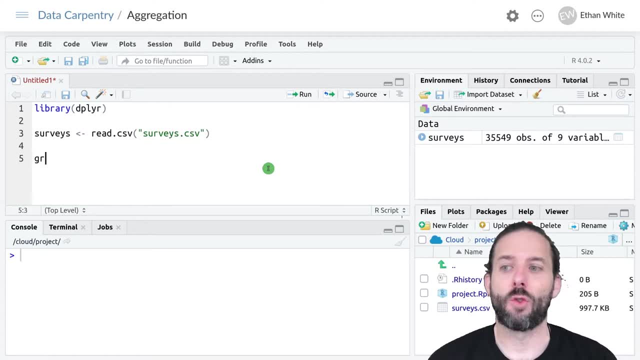 And we do this using the function groupBy, And that function's arguments are first, the table we want to work on and then second, one or more columns to group by. And so let's go ahead and groupBy speciesId, So we'll give it the name of the table that we want to work on, the Surveys table, and 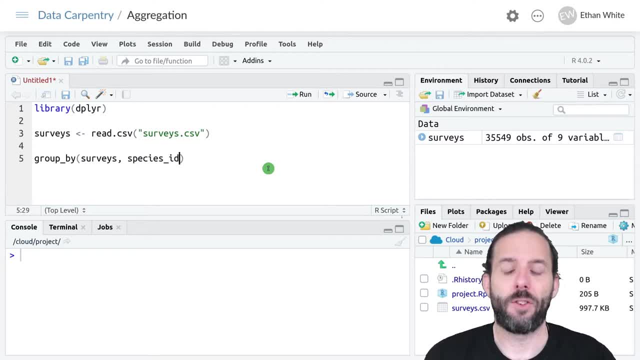 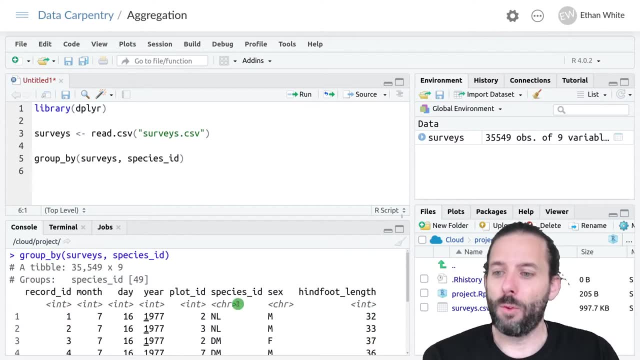 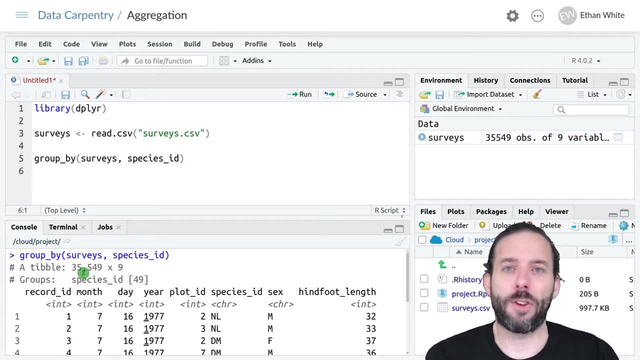 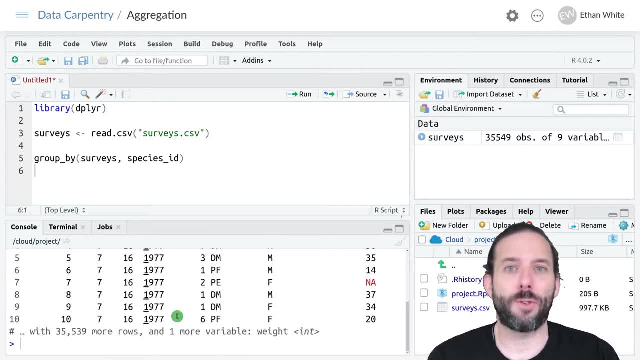 And it's telling us that that tibble is grouped based on the speciesId column and that there are 49 groups. These data frames also look a little different because they only print out the first 10 rows to the console, which is nice. we have less scrolling and it tells us about the data. 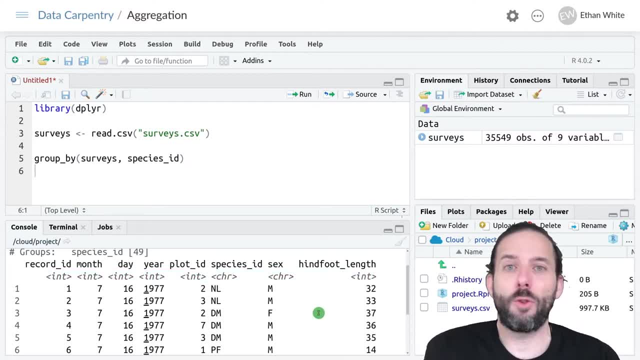 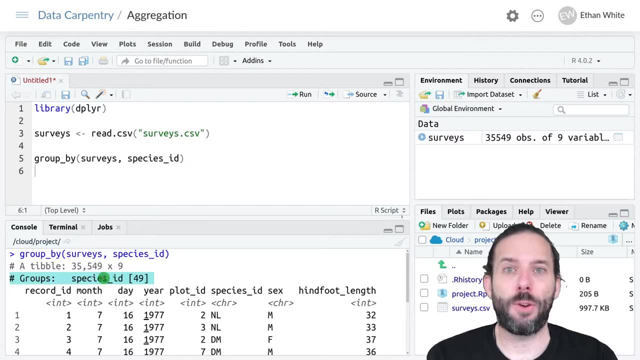 types in each of the columns. But for most purposes this will work just like an ordinary data frame and by having groups, it will allow us to do the next step in summarizing the data. Let's go ahead and store this data frame so that we can use it in the next step. 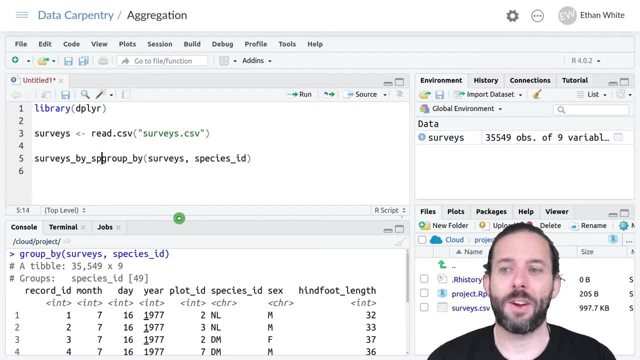 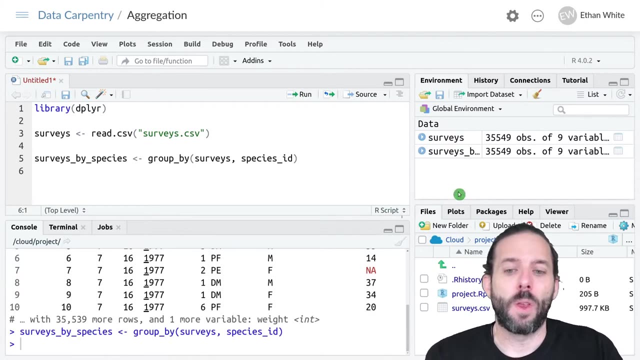 And we'll call it surveys underscore by underscore species, since it's surveys grouped by species, and then we'll assign the results of this group by to it, using the assignment operator. If we run this, we'll now see that we've stored that table. 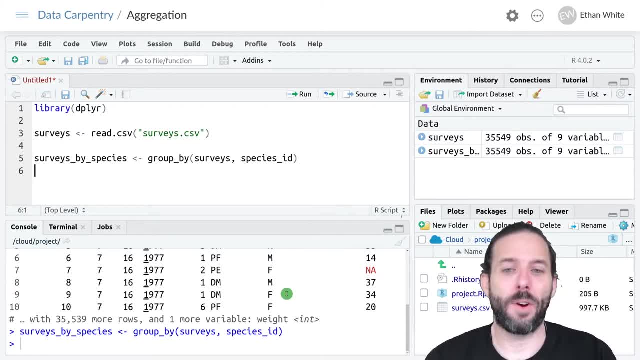 Or tibble, as a variable so that we can use it. After grouping our data, the next step is to summarize it using the summarize function to calculate whatever value that we want for each group in that table. So let's start by counting the number of rows in each group, and we're going to do that because 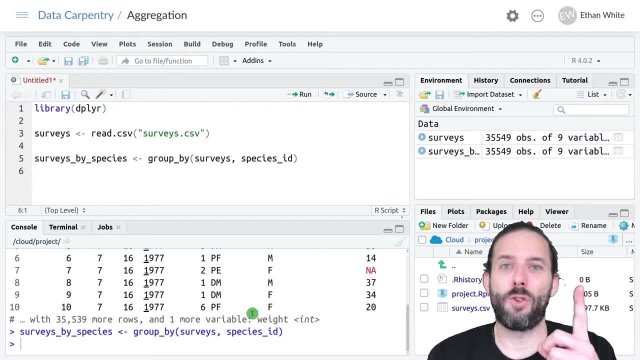 each row in this table represents one individual small mammal, and so by counting the rows we'll get the number of individuals that have been captured for each species, And we do this using the function summarize, And the arguments for summarize are the table we want to summarize and that needs to be a grouped. 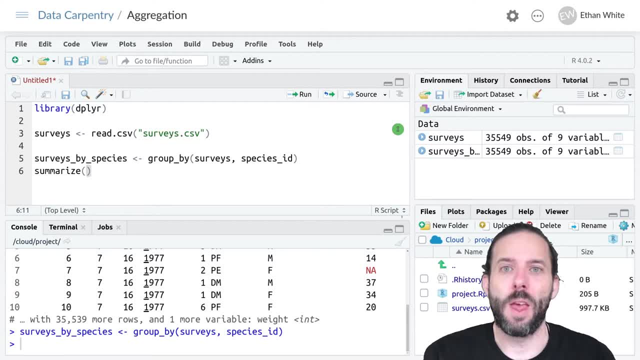 table so that it can do the summary for each group. So we'll also calculate the number of circles If we run these and select theре palace and these terms at the top and then the termMINI totally glass or in other verses. by the way, 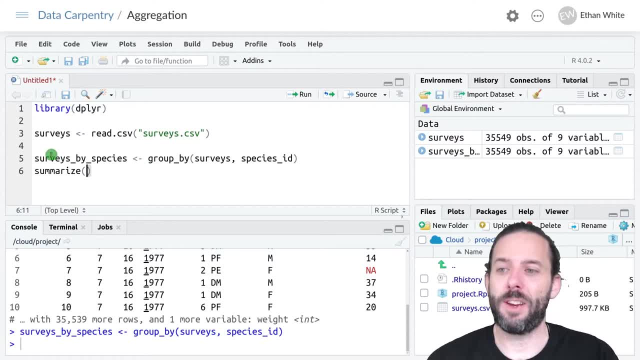 is literals andénery, then we're going to simply orphan this off into the reariascule table. so this is the grouped table that we want to work with. So surveys by species comma, And then we want to count the number of rows, because that's the number of individuals, And so 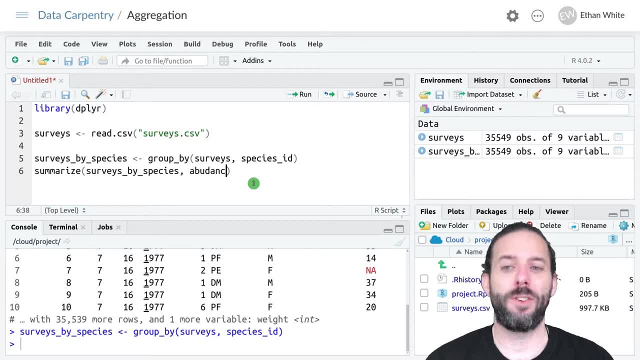 we'll call this abundance. That's another way that we describe the number of individuals, And I will spell it correctly with the N. So that's going to be the name of our new column, And then an equals sign And then the calculation that we want to do And to 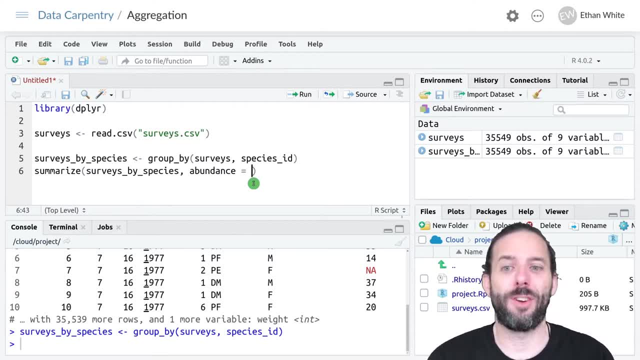 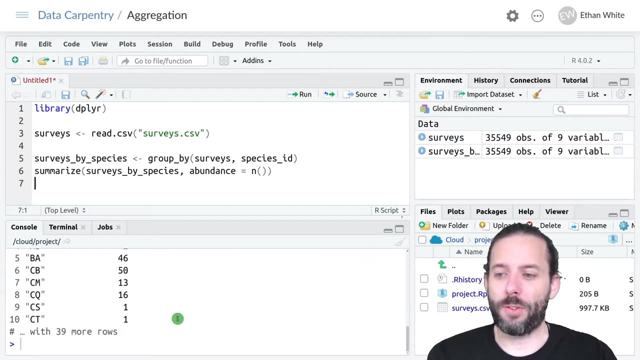 count the number of rows in the table. there's a special function called N or number, And it's a function, so it needs parentheses, But it doesn't have any arguments because it's going to apply to the whole table And if we run this code, 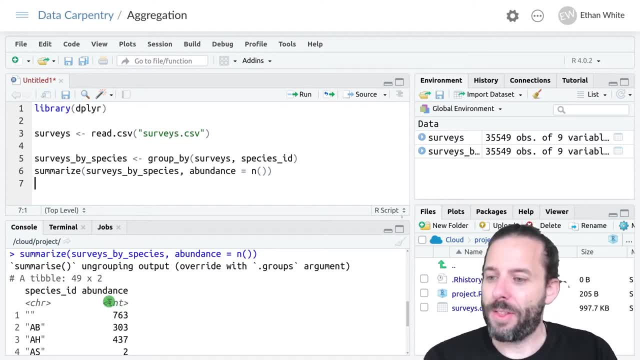 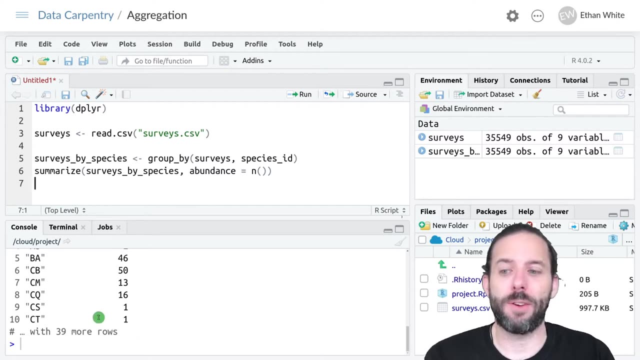 we can see that we have a column with the species IDs in it and another column with the counts of how many individuals of that species have been seen during the entire period of the study. We can also group by multiple columns. So let's say we wanted to count the number of 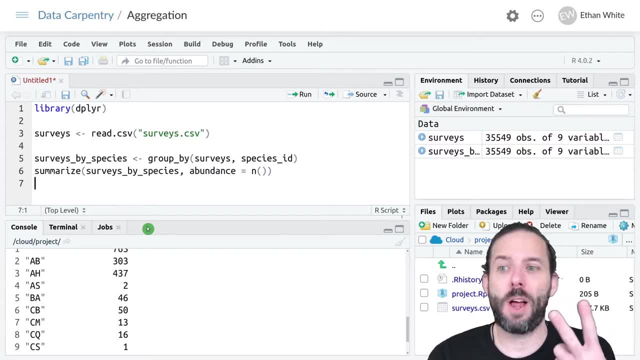 individuals in each species on each plot. To do this we need to go back to the group by step And group by more than one thing. So let's call this surveys by species plot, to indicate that we're grouping by both of those. 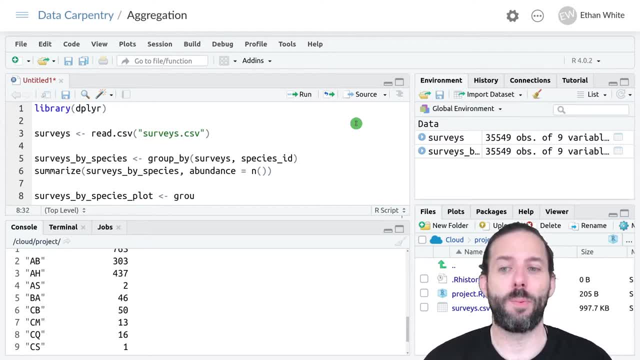 And then we're going to assign to that the results of the group underscore by function. Again, we're working with the surveys table. We still want to group by species ID, But Now we also want to group by plot. so we'll add another comma and then plot underscore. 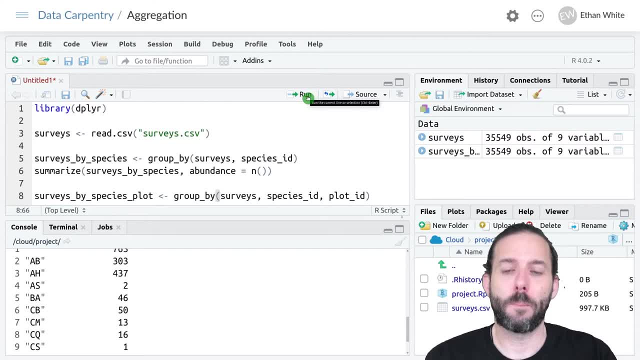 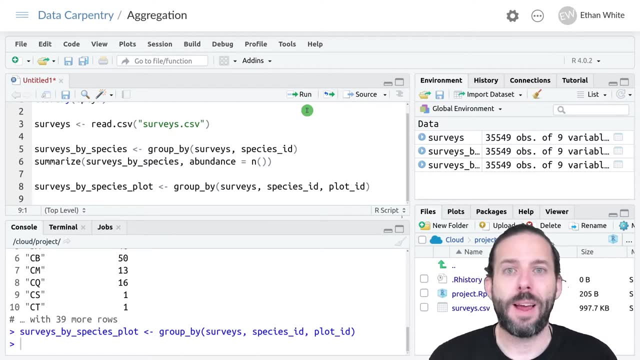 id, because that's the name of the plot column. We then run this to do the grouping. Now that we have our new data frame grouped by two columns, we go ahead and run our summarize command on that data frame. So summarize- parentheses, surveys by species, by plot, and then we do the same calculation. 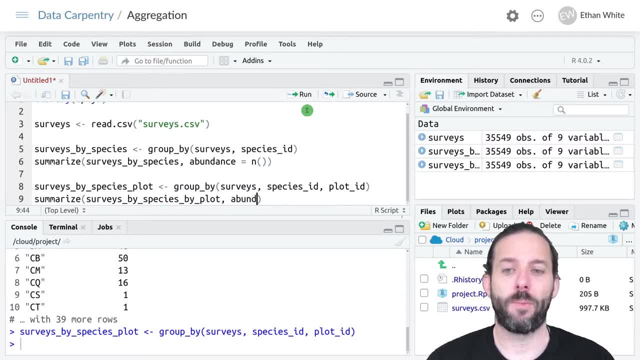 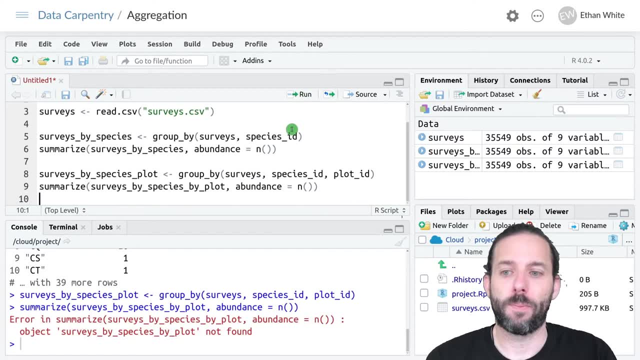 we did before. so abundance equals n and parentheses, And it looks like I've made an error. Surveys by species by plot: not found. I called this surveys by species plot. I added an extra by here, so we'll go ahead and take that out and then rerun. 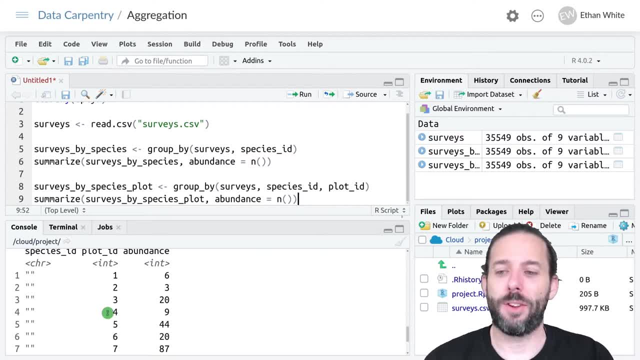 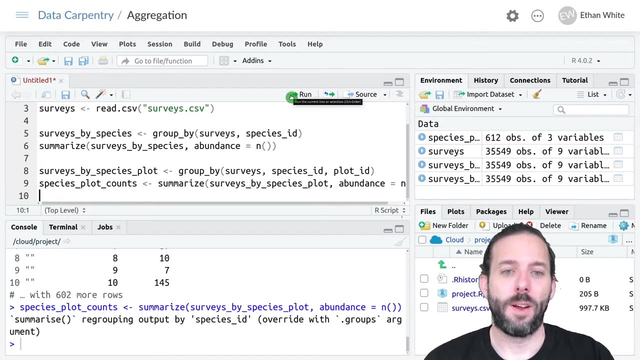 And we can't totally see what's going on here because we've only got 10 rows. So let's store this in a variable called species plot And then run it, and then we can come over here and look at what actually happened above. 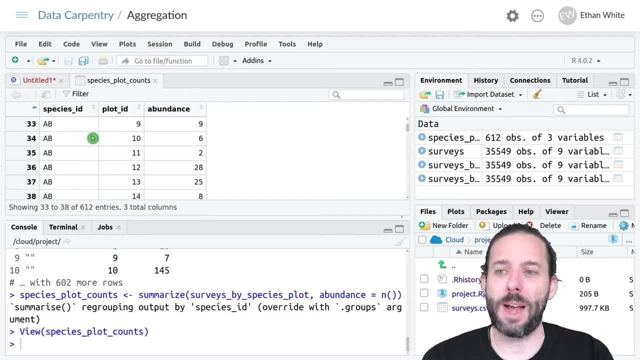 We have some null species IDs which we don't really care about, but then we can see that for each species ID and each plot. So this is species AB. on plot nine, There were nine individuals and it's done this for every single species and every single. 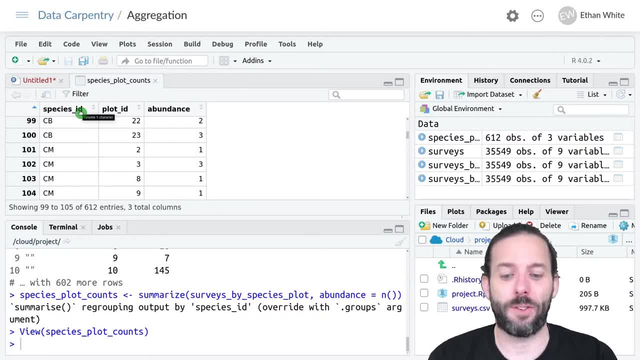 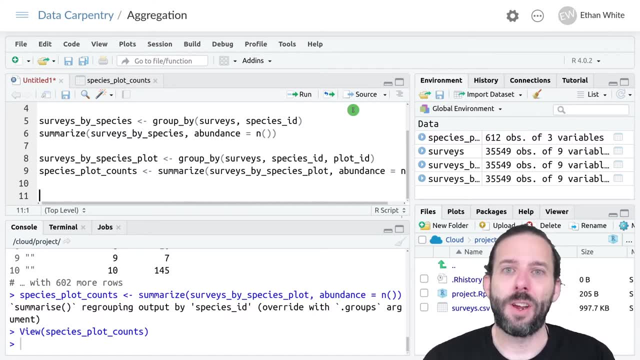 plot. We've got this nice summary that's ready for analysis, And we're not restricted to just counting things. in fact, we can do any calculation that involves functions that take a vector and return a single value. And so let's go back to the example that I mentioned at the beginning, where we want to 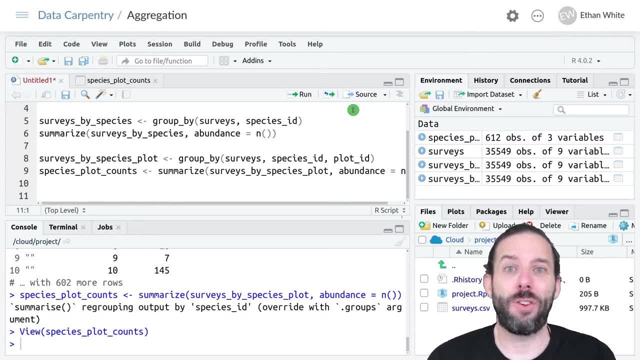 calculate the average weight of each species on at the site, And we can do that using summarize. So let's go ahead and create a variable to store this in. We'll call it species weight And then to that we'll assign the output from summarize. 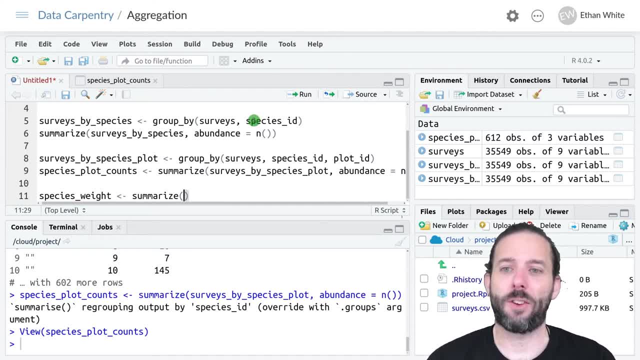 We're just grouping by species. so we'll go back to the surveys by species variable that we created- Surveys Underscore By And under Underscore Species, And then now to calculate the average weight we need again the name of the column that. 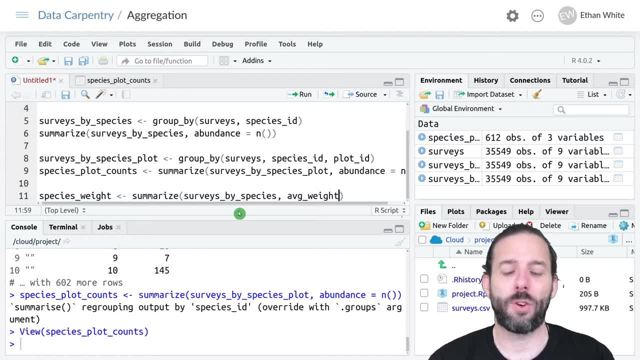 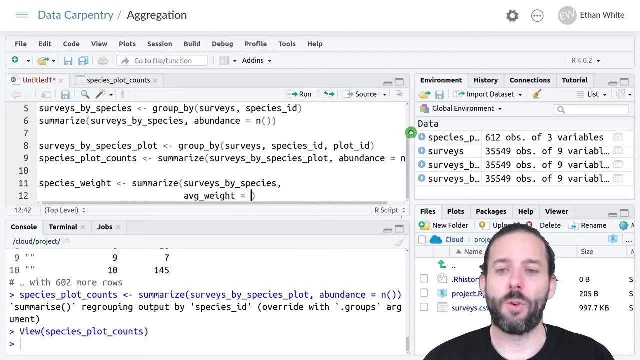 we're going to create, So we'll call it average weight Average under AVG. underscore weight disappoints- Wait, equals- and then the calculation that we want to do. I'm going to move this down to the next line so we can see it clearly, and so we can now. 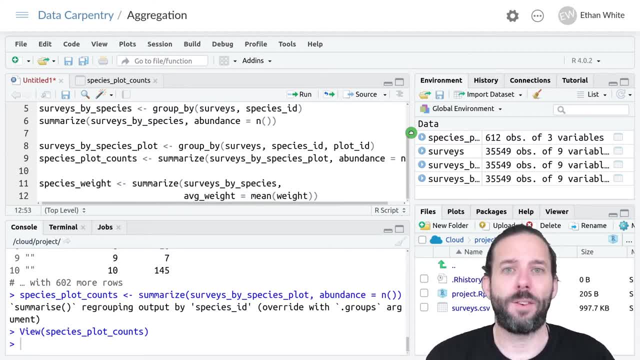 say the mean of Grade Of Every weight. and so what this will do is, for each group, which in this case is a species, it will take the weight column, calculate its average and store it in a column named average weight. and if we run this, we can then go over here and 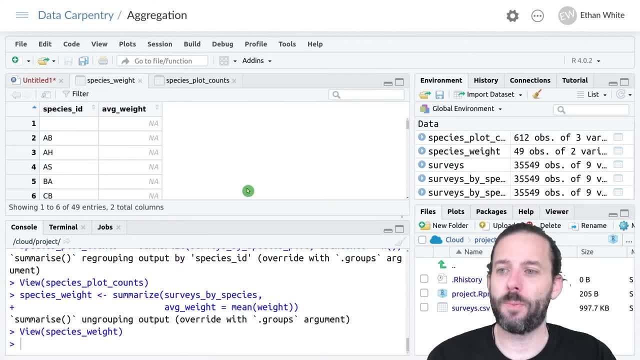 look at the species weight table. that results: oh, that's interesting. now we have each species ID, but all of our average weights except for this one, except for a few, are null. why do you think that might be any ideas? if your answer was that when we take a mean, if there are any null values, 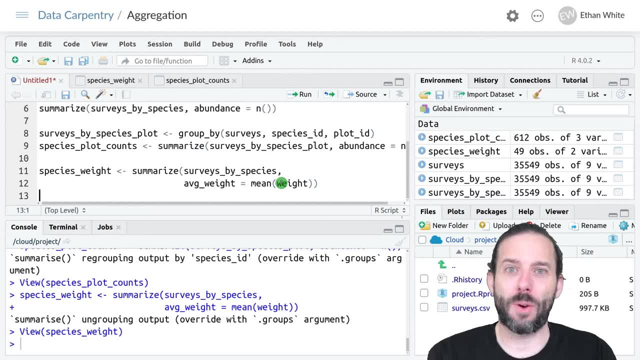 we get back our c position. Let's go inside of our j array a null value as the result. then you're right and if you remember from a couple of weeks ago, we can remove those nulls before calculating the mean by adding an optional argument to mean, and so we put a comma and then na dot RM equals true. 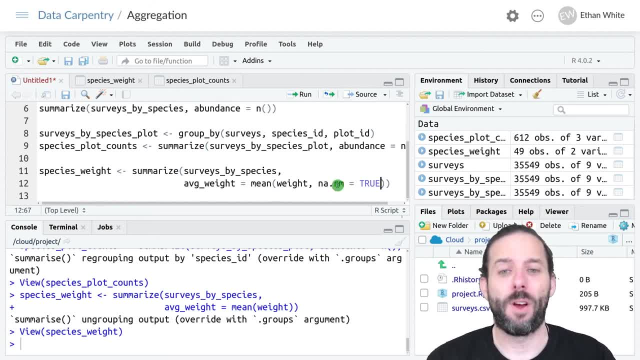 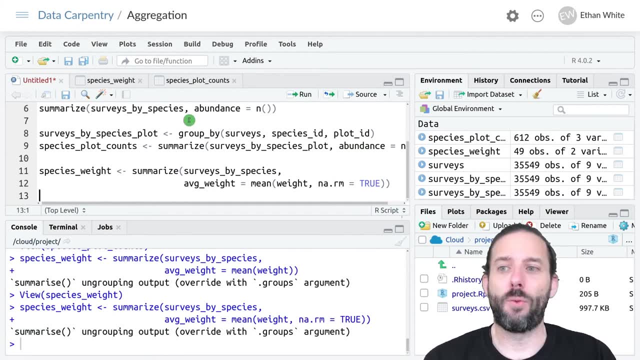 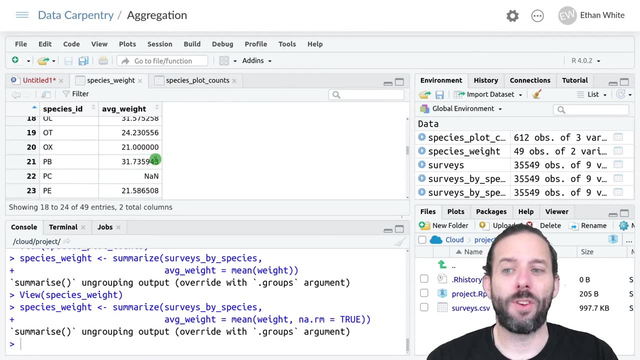 which tells it to remove all of the null values before calculating the mean, and so if we rerun this and go back to the species weight table, we'll see that many more of our species have average masses. now there are still some nan sticking around, and those are there for species that have never been weighed, and so 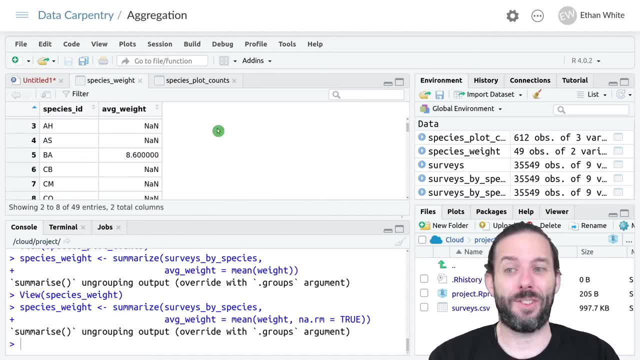 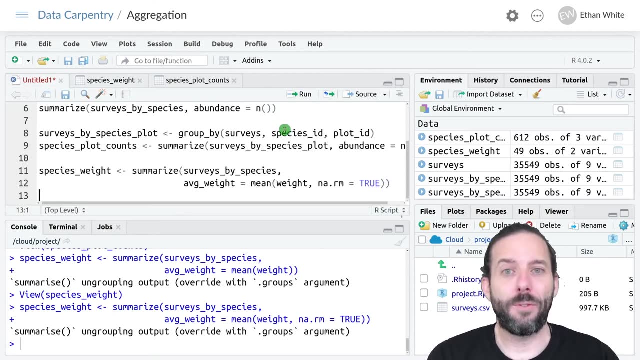 these are things like birds, birds, birds, birds that get into traps, snakes that get into traps, certain kinds of mammals that we don't weigh at the site, and so those are just. there's no data there to calculate a mean for, and if you wanted to get rid,